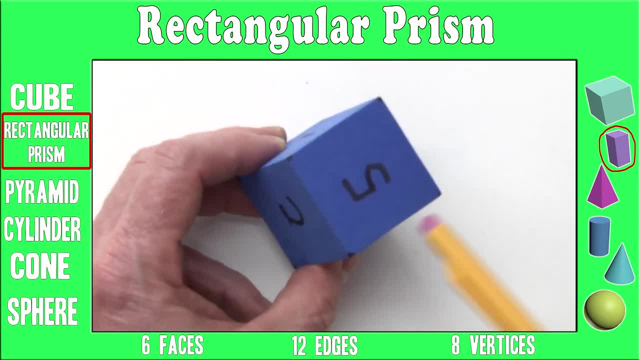 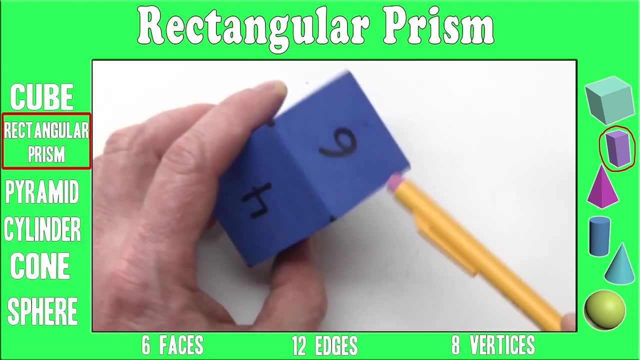 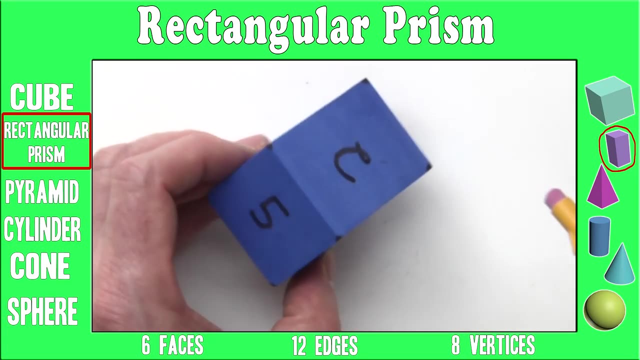 prism has twelve edges: One, two, three, four, five, six, seven, eight, nine, ten, eleven, twelve. A rectangular prism has eight vertices: One, two, three, four, five, six, seven, eight, 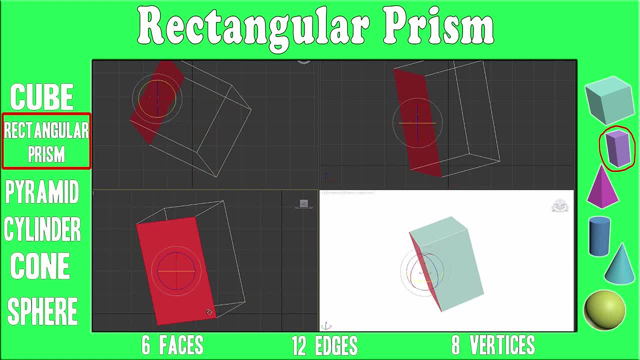 A rectangular prism is like a cube, but just longer. Same number of faces, edges and verifications. It is generally said that if you have a squareying prism you can make it like this. So one, two, three, four, five, six, seven, eight. Using our 3D program, you can see that the 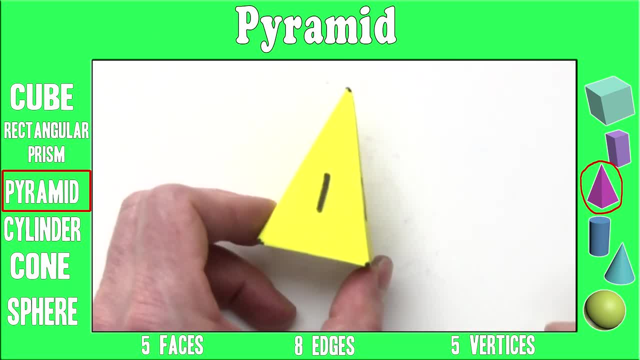 cube has five faces: One, two, three, four, five, nine and six. This is an edge. A pyramid has five faces: One, two, three, four, five, eight, nine, ten, nine, nine, ten, eleven. 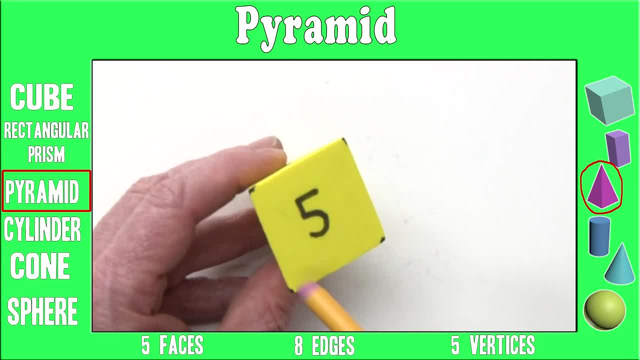 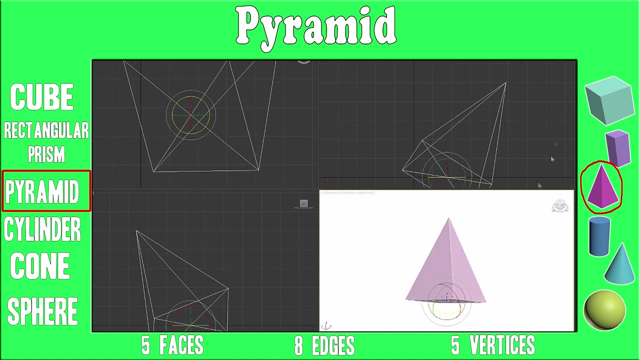 A pyramid has eight edges: One, two, three, four, five, six, seven, eight. A pyramid has five vertices: One, two, three, four and five Pyramids are the same shape as a pyramid in Egypt. 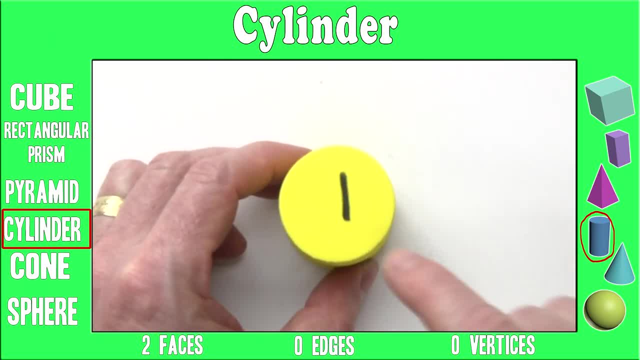 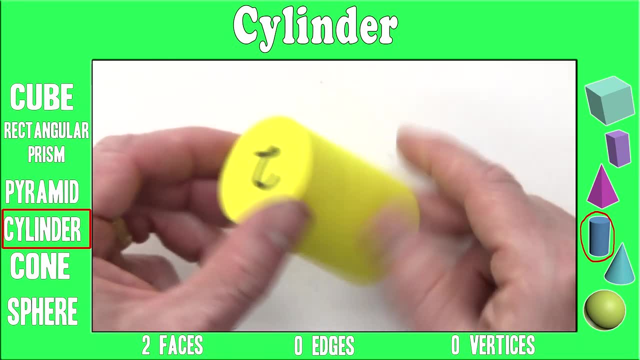 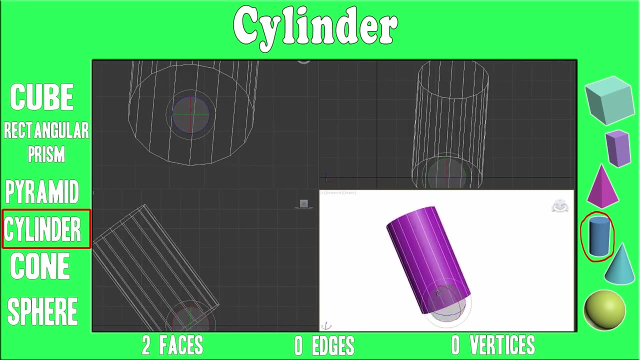 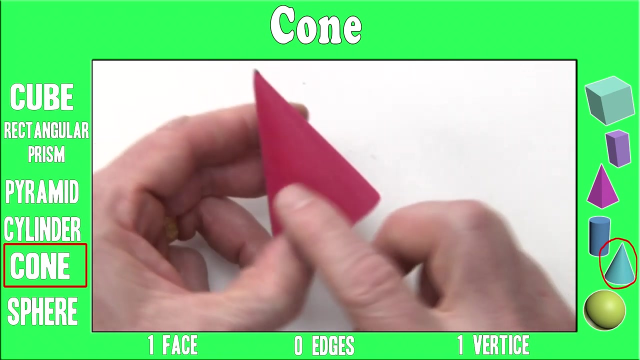 Cylinders have two faces: One two. They have zero edges and zero vertices. For this lesson: we only count flat faces, not curved faces. A cone has one face, zero edges and one vertice. A cone reminds me of an elephant. 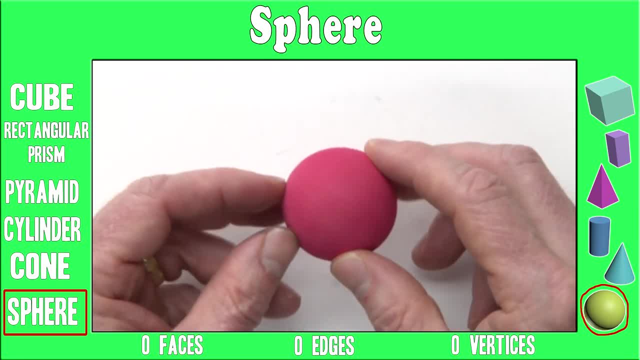 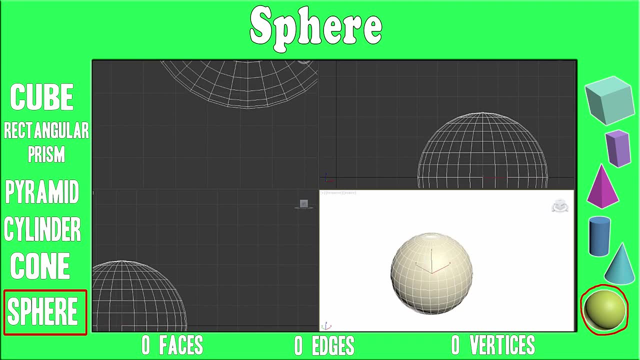 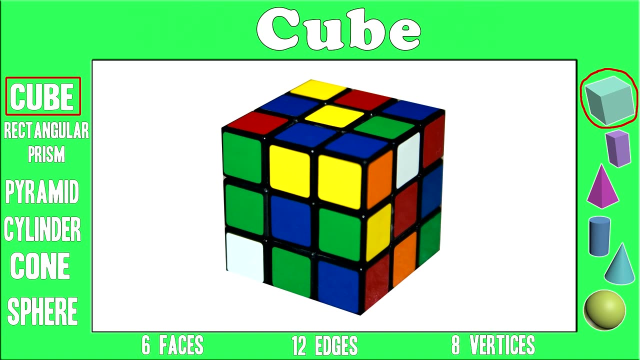 An ice cream cone: Yummy Sphere. Zero faces, zero edges and zero vertices. A sphere is like a ball, So let's review. What shape is this? You're right, It's a cube. What shape is this? 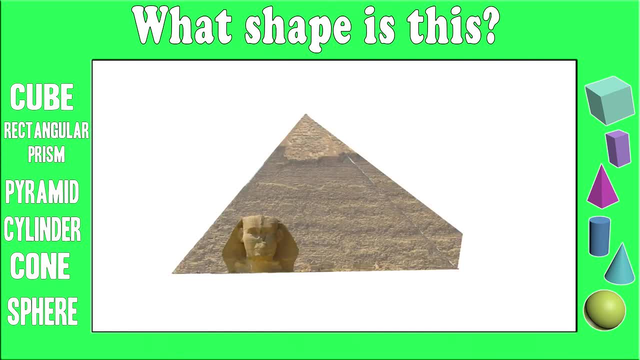 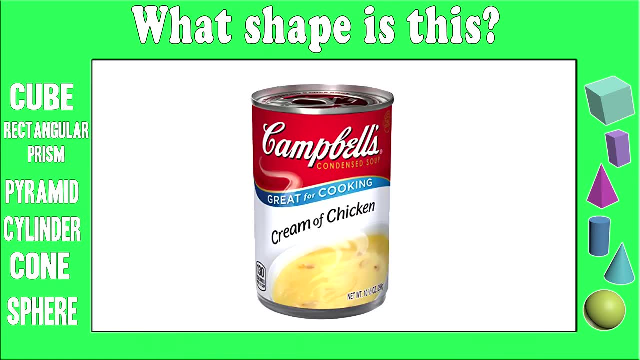 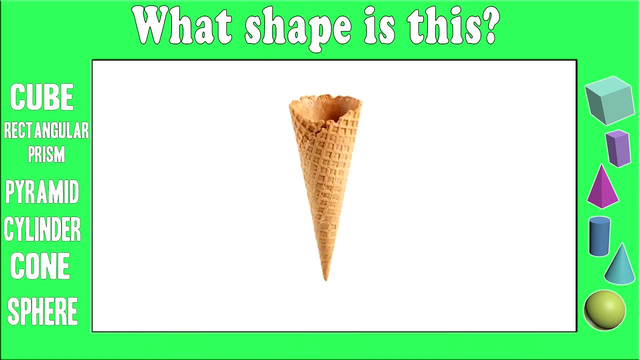 Excellent. It's a rectangular prism. Now, what shape is this? Perfect? It's a pyramid. What shape is this? Correct? It's a cylinder. What shape is this? You're right, It's a cone. What shape is this? 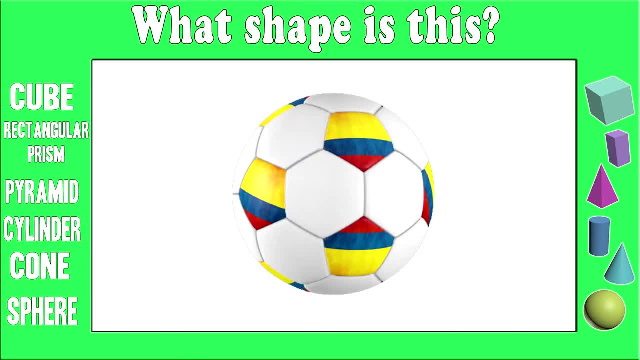 Excellent, It's a sphere. Hey. thanks a lot for watching the show today. I hope you had a fun time learning about these different 3D shapes And make sure you check out my other videos on here. I have a lot of cool educational and art videos.